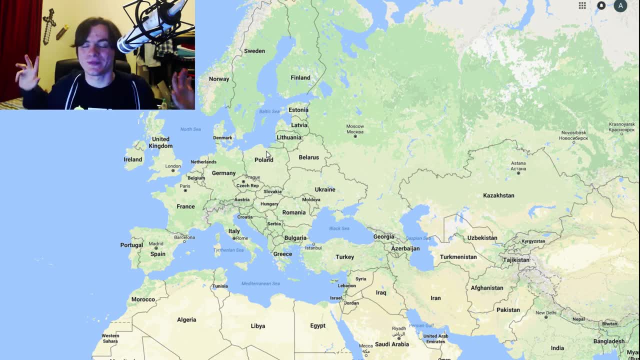 Hopefully, you all do enjoy it. With that said, though, let's get straight into it. This is kind of a big topic because, again, there's 51 countries in Europe. There's like 61 languages I want to say. 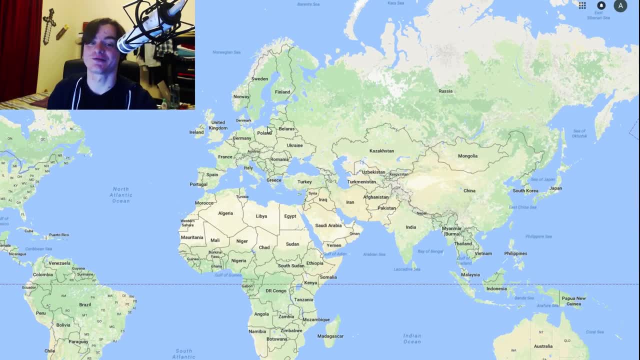 There's a lot of stuff to go through, But let's try and start with the first bit, which is the Outreges. Let's work from the outside in, shall we? And basically, the Outreges of Europe are Iceland. 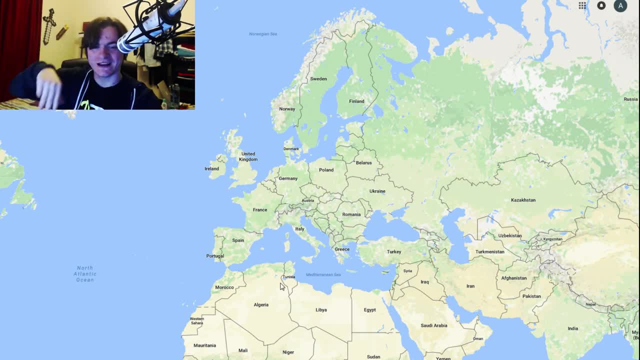 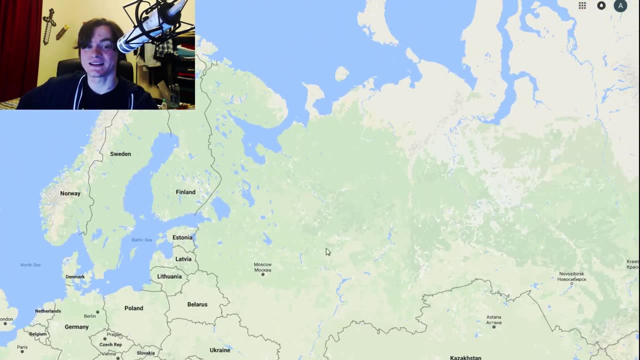 So this is the Outer Edge and, like the Northwest side, The Southwest Edge would be like Portugal, The Southeast Edge would be somewhere in the Caucasus region, like over here It cuts through a little bit of Kazakhstan, And then the Northwest Edge is somewhere in Russia. 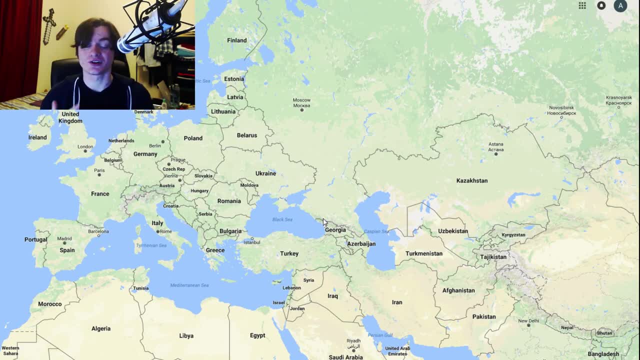 So yeah, it's kind of like a box like that. because the definition of continent changes so much from continent to continent, It's kind of hard to say what is and what isn't. You can kind of get different definitions, But for the most part some of Turkey is cut off through there. 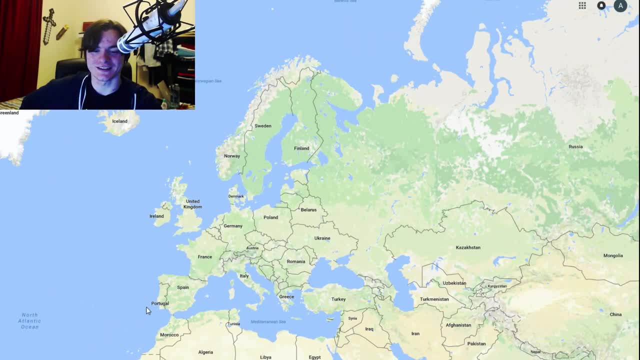 And yeah, there's your rough Europe right here. So let's show it with my mouse, just like this: You cut through Turkey, Then you take the Caucasus. anyway, You don't take Iran, You take a little bit of Kazakhstan. 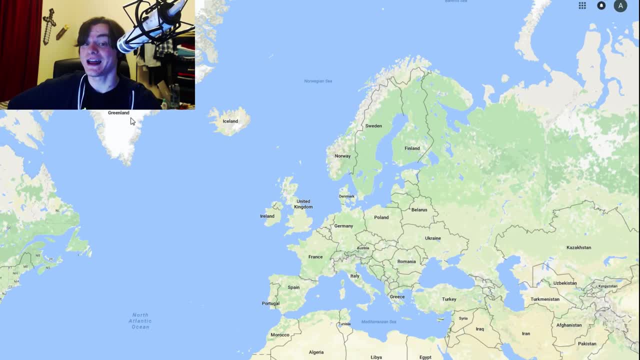 And then you call that Europe. That's Europe right there. That's great. And Greenland is not part of Europe for a lot of technical reasons, But because it is part of the country of Denmark, you can kind of consider it a European country. 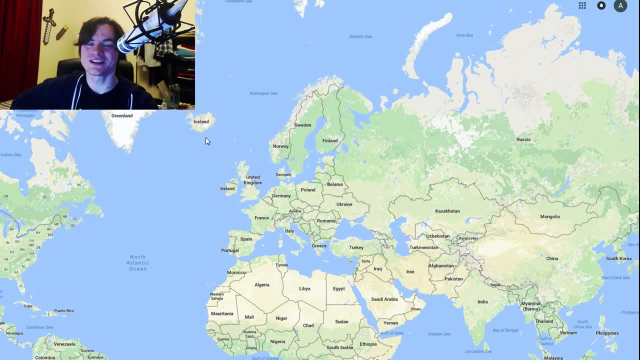 Again, it's weird, They're different, It's not really, But yeah, there's your edge of Europe. Now you know, Let's first go through the like. I guess the transcontinental countries, The ones that are European countries but mostly don't exist in Europe. 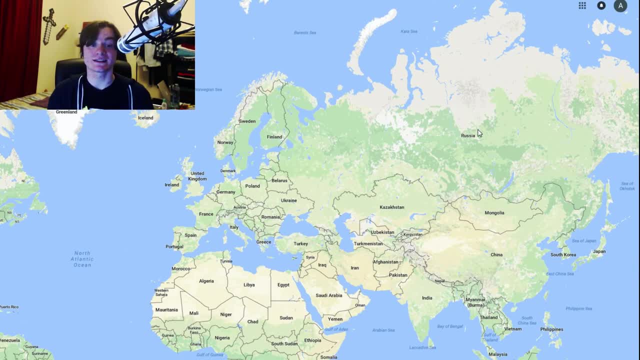 So, first of all, the most notable is Russia, right, So Russia, Russia, biggest country on Earth by landmass, like by a lot, It's giant. Look at the size of Russia. It's in Europe, It goes all the way through Asia. 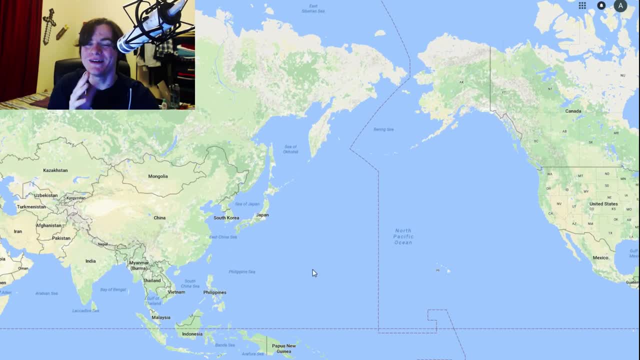 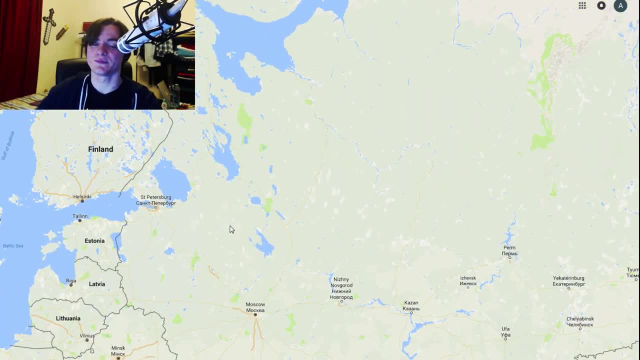 So now you know As well as one of their second biggest cities, I think it is St Petersburg, Both inside Europe. Next up we've got Kazakhstan. Again, a little bit of it gets cut off by Europe because of our definition. 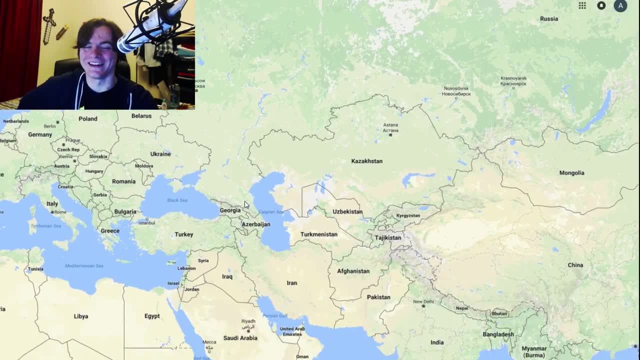 So Kazakhstan, European country- technically Not really, though I mean You can kind of count it as one- And then Turkey is the same deal, where only 3% of Turkey exists in Europe. This little part right here. 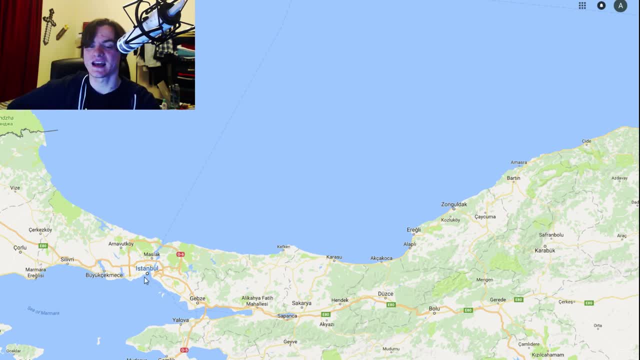 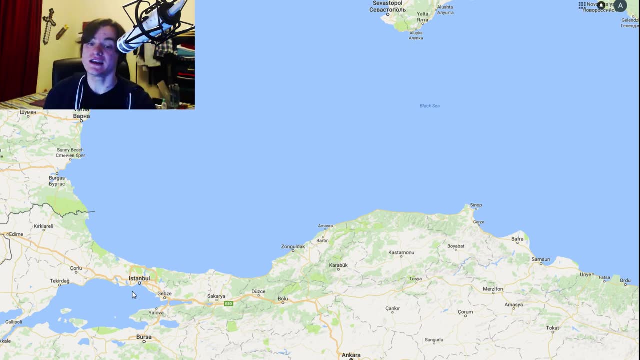 In fact, Istanbul, one of the biggest cities, Yeah, Turkey's biggest city- is cut off by, you know, the Europe-Asia divide. So some of Istanbul exists in Europe And some exists in Asia. So, yeah, this is kind of like the gateway to Asia. 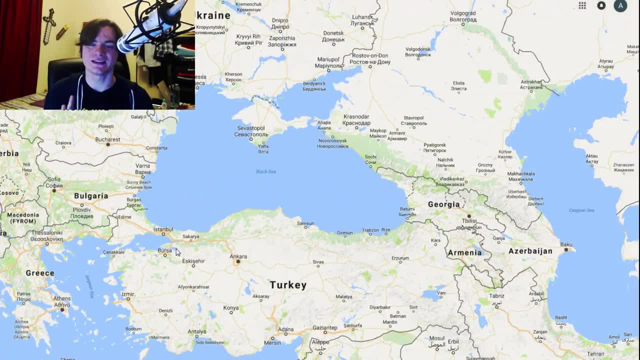 It's often called, And yeah, it's one of the biggest cities in Europe- Technically the biggest if you count the Asian side, which is where things get confusing. But yeah, there is Istanbul right there, One of the other edge points of Europe. 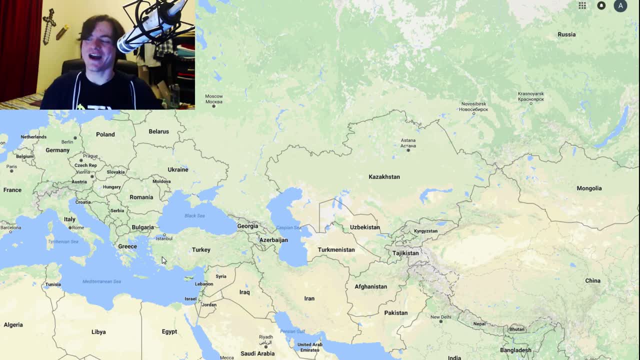 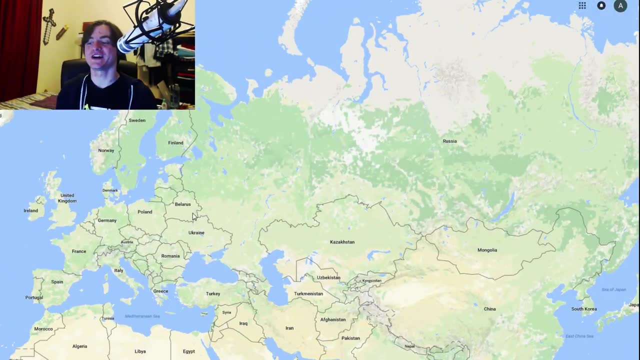 And also the third of the, you know, the transcontinental. So now we're down to like 48 real European countries where they all exist there Or most exist there, And let's just get straight into it with, I guess, the one everyone's heard of right. 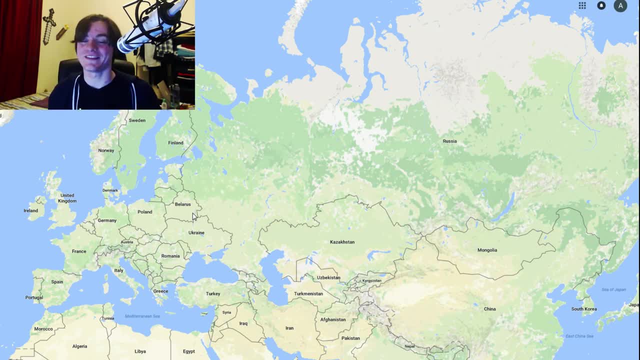 Because everyone has heard of Scandinavia, Everyone loves Scandinavian, this or Scandinavian- that They're all friendly, They're lovely, They're very, you know, like I guess- wealthy relative to the rest of the world, And they're also very nice. 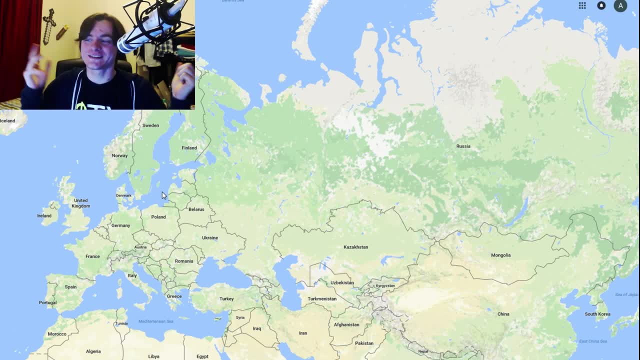 And they speak English. It's all lovely And everyone's heard of it, right? Well, I hope so. If you haven't heard of Scandinavia, then I don't know. But yeah, Scandinavia, are these three countries right here? 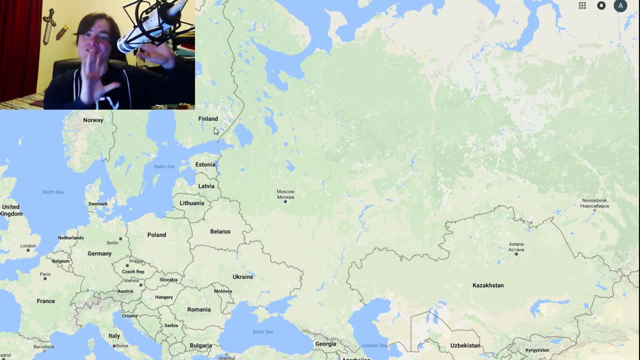 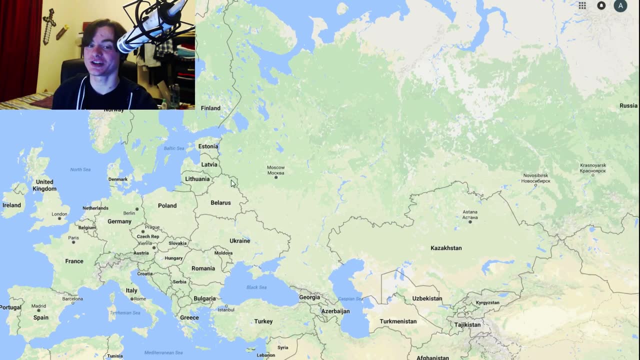 Sweden, Norway and Denmark. It does not include Finland, even though Finland's like awkwardly to Norway and Sweden. That is a part of a separate definition called Fennoscandia, which no one really ever uses. But yeah, this peninsula as a whole is called the Fennoscandia Peninsula. 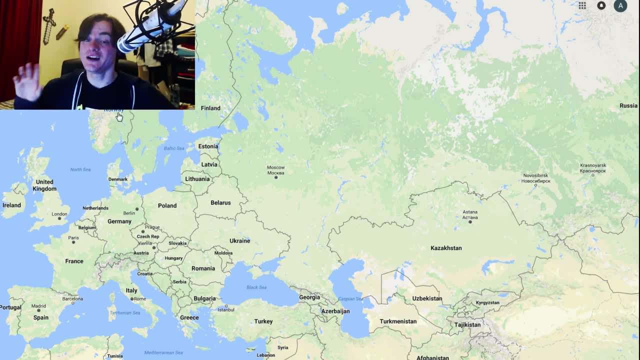 No one ever calls it that, though. There's Scandinavia right here, which is what you need to know. However, there's then a second definition called the Nordic countries, which includes Denmark, Norway, Sweden, But then Finland gets to join in on the fun. 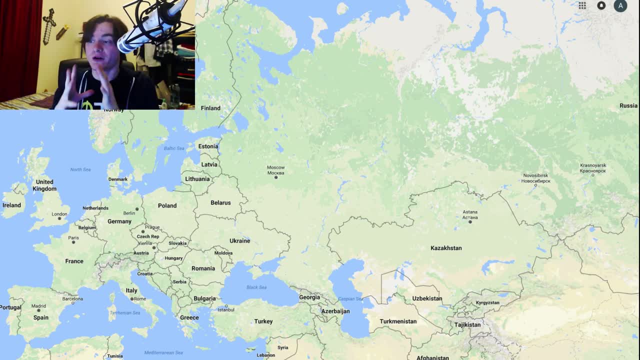 Again, Finland is kind of like: you know, Sweden, Norway and Denmark are very, very close and like countries. Finland's like that. but then it's an extra step removed. I'd say: So yeah, Finland becomes part of the Nordic country definition alongside 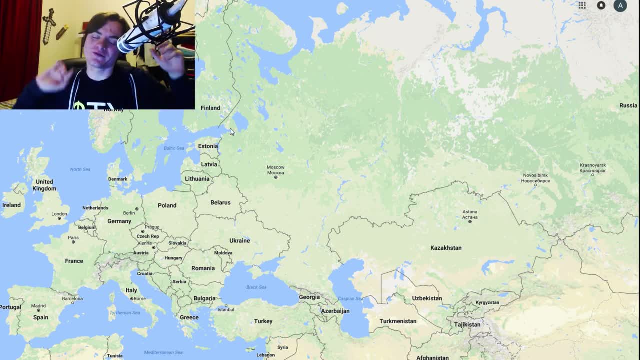 Iceland, and these five are the super north. you know, when you picture a Nord from Skyrim or whatever or whatever you want to do, that's kind of what they're called. And if you're curious as to why they're called Nordic or Nord, it's because I believe that's one of the Scandinavian words for north. 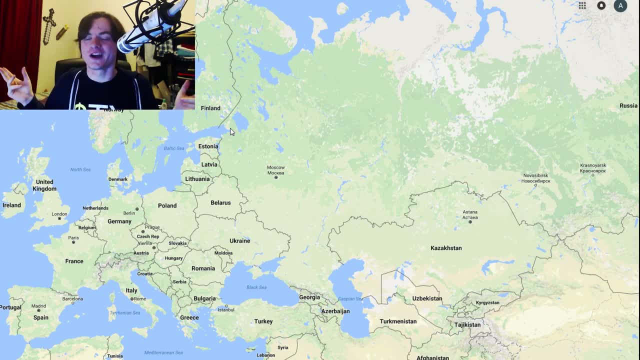 you know the Norden, it becomes Northern. So yeah, they're Northern countries. It's basically Northern Europe, but they're called the Nordic countries because Northern Europe can then contain the United Kingdom sometimes and also then contain the Baltic states. 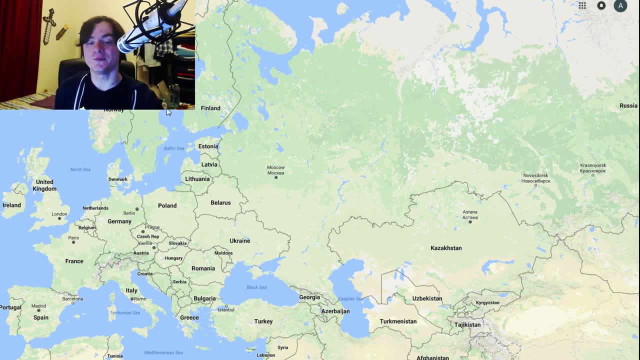 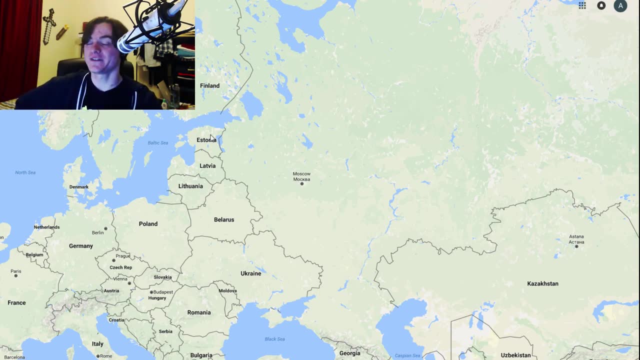 So yeah, the Baltic states is the next easy one to go through. The Baltic states are these three right here? They used to be USSR Republic. They really didn't want to be The moment they could go free. they did, and there's three of them. 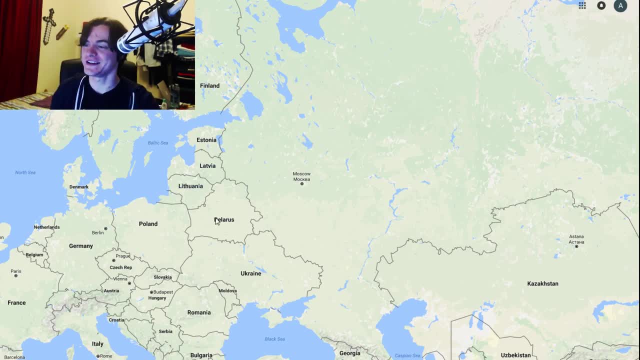 There's Estonia, there's Latvia and there's Lithuania. So these three right here they're called the Baltics and they're all kind of friends. Lithuania wants to be more friends of Poland and call themselves Central European. Estonia wants to be a Nordic country, but for the most part you just need to bear in mind these three countries right here. 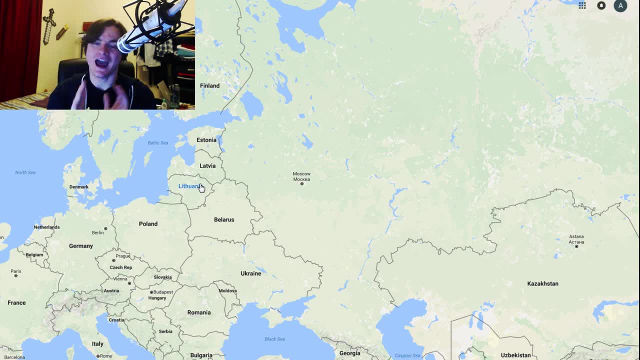 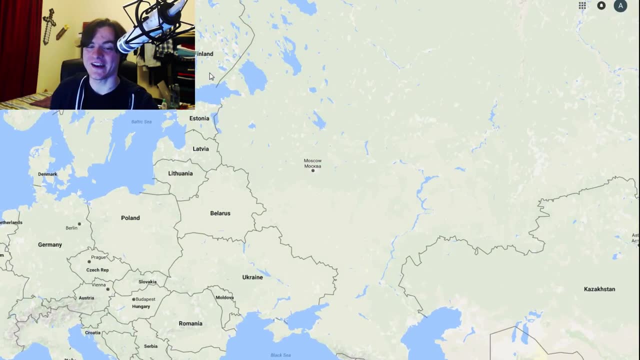 They're, all you know, Baltic and they have lots of very close ties together and they're kind of similar. Again, we're just trying to separate Europe into regions right here. So we got, like you know, Scandinavia, Nordic countries, and then over here we've got the Baltics. 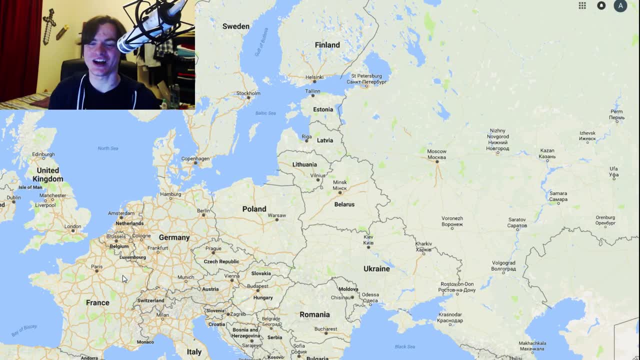 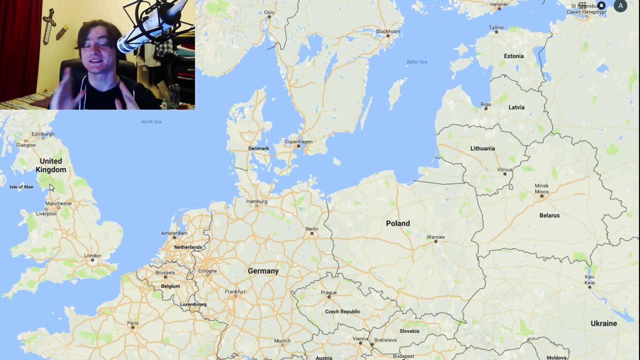 So boom, That's, that's it. That's like North Europe covered. besides the UK and the British Isles, which you know for now, let's just say British Isles are the United Kingdom of Great Britain, Northern Ireland, which is this country right here that you have to get a whole video from, because it's such a mess of stuff. 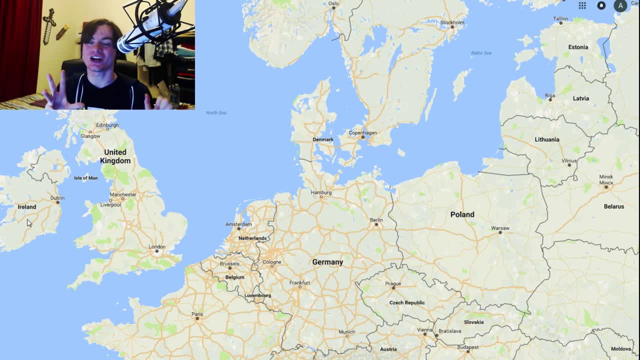 But yeah, the United Kingdom right here. and then also there's Ireland. Those are called the British Isles. They're technically a part of Northern Europe but, depends on your definition, They're definitely part of Northwest Europe, alongside Iceland. so there you go. 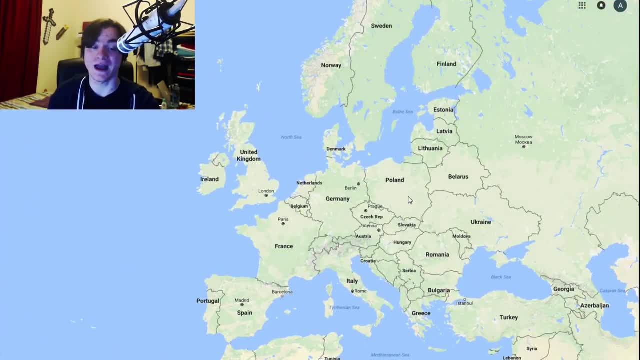 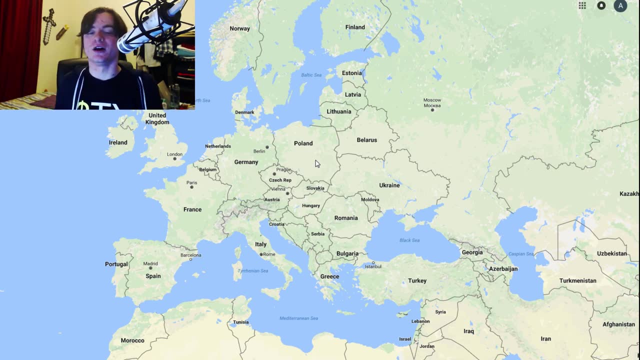 There's. there's your Northern Europe, current. So let's go- now you know, down from that to the West of Europe, because Western Europe is what I would really describe as like the Europe everyone visualizes and wants to visit for the most part, because Western Europe it's generally kind of picked at the 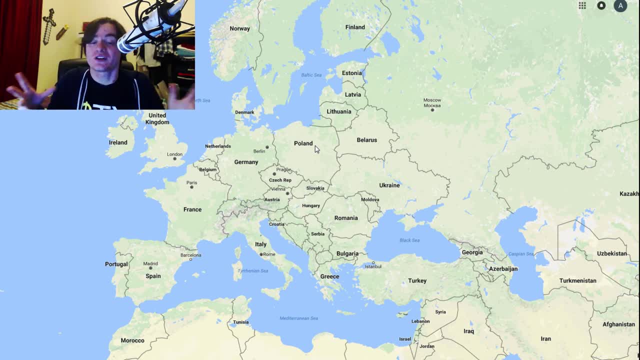 what's it called the Iron Curtain Line, the line that was divided, you know, for most of the Cold War. you know the fighting ground of that because, yeah, if you look at Europe, for the most part the Western Europe side is divided, right down here the Germany-Poland border. 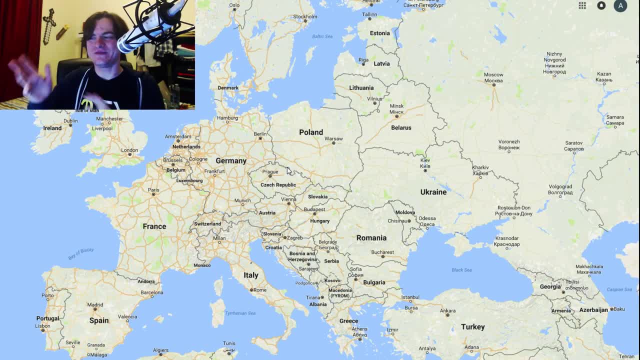 because, again, Poland was part of Warsaw Pact and Germany, most of Germany anyway- was, you know, part of the whole NATO. I think, Yeah, NATO, I guess it'd be, And basically yeah, so Western Europe is most most of this right here includes Austria sometimes. 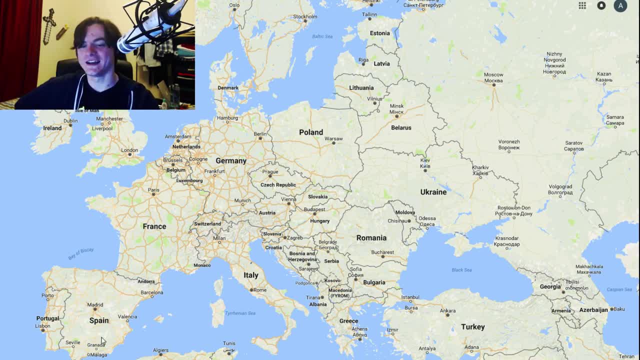 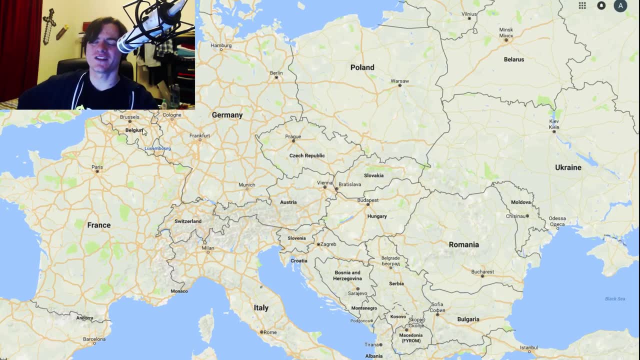 whatever you want to do, but it kind of cuts across here. It's France, Germany, the UK, Spain, Portugal, Italy, etc. And, yeah, these are generally the- I guess, the richer countries in Europe. They're also the ones that contain a lot of the bigger, well more known sites. 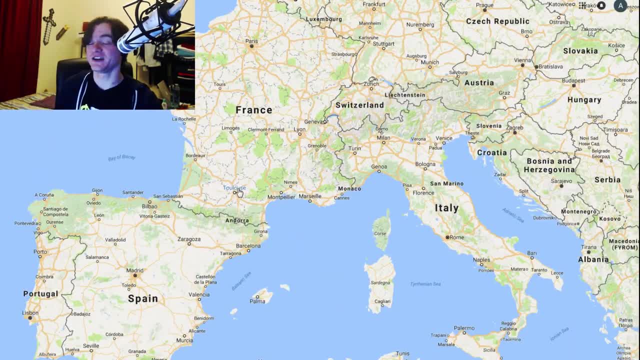 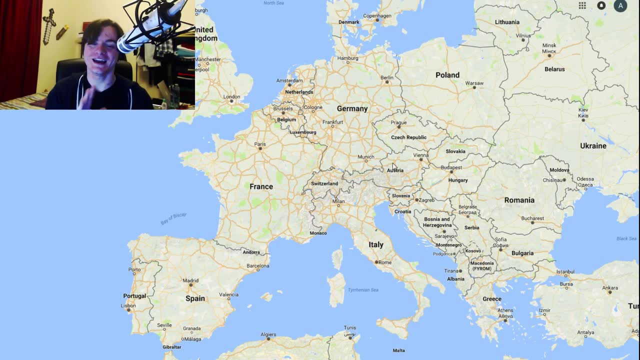 such as Amsterdam, Berlin, Paris, Barcelona, you know all the the pretty luxurious European cities, Rome of course, and that's that's Western Europe, right there. Again, it gets a bit more complex than that because there's also South, South Europe. 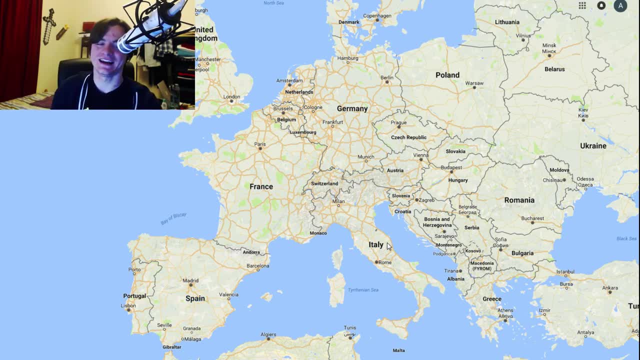 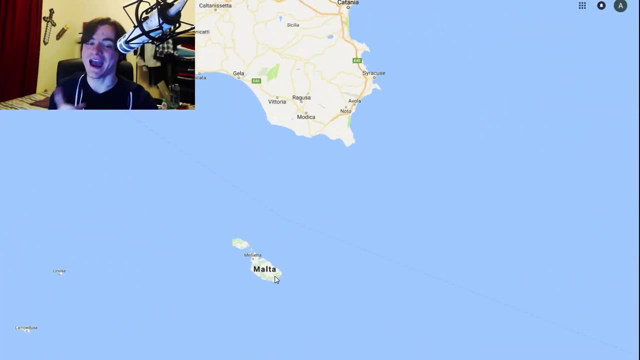 which includes some of Western Europe. So South Europe is Spain, Italy, Greece, sometimes Portugal, sometimes the island states of like Malta over here. so I always lose Malta on the map. and here's Malta, right here. Then, as well as you know the fact that we've got like, okay, we've got South Europe, 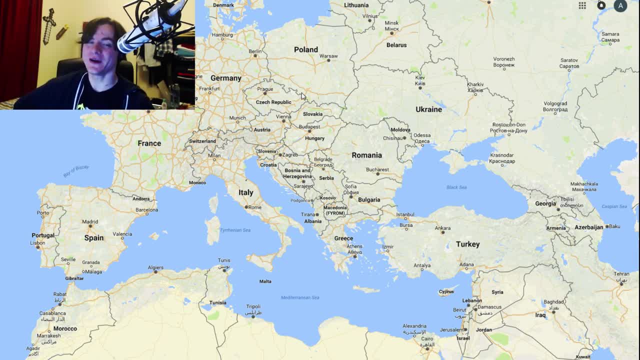 we've got West, we've got North, we've got all that stuff covered. so is the rest just Eastern Europe? Well, sort of well. here's the thing right, because if you look at you know Europe on. 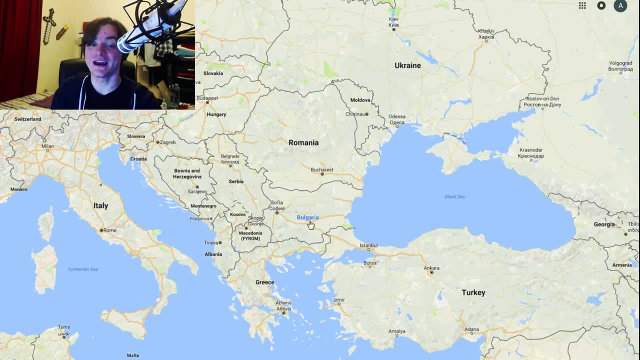 a map. you actually kind of get into the mess thing right here because there's just a giant mess of countries right here and the long story short on that is that they used to be very close together and they split as recently as like 20, 30 years ago. so you generally 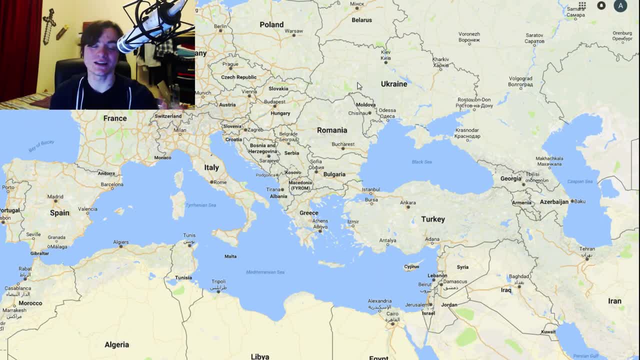 kind of call this like South East Europe and you call that East Europe. There's a lot of overlap, but let's just go straight into it with the Balkans right here. so you know, after you've sorted out past that, you're like, okay, there's lots of countries. 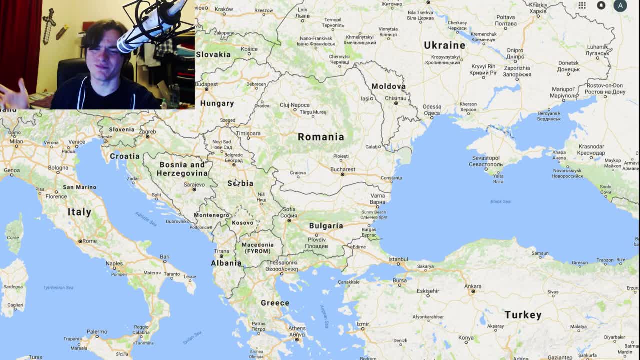 here The Balkans are anything in in the, I guess the Balkic, uh, Balkic, that's not it at all. but yeah, the Balkans are these countries. right here, we got the Slovenia, we got Croatia. 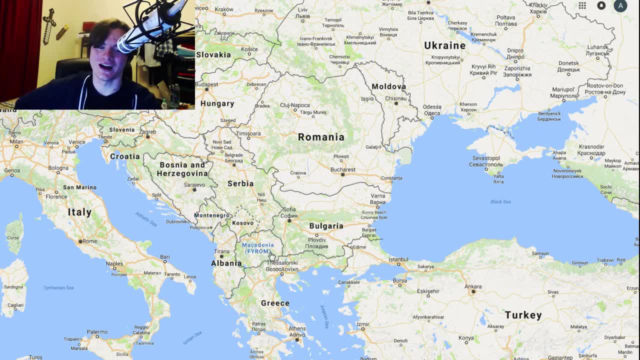 we got Bosnia, we got Serbia, we got Montenegro and we got um Macedonia or the former Yugoslav Republic of Macedonia. their name causes a whole bunch of controversy because um Macedonia is a Greek thing and basically, yeah, FYR, or whatever you want to call it. 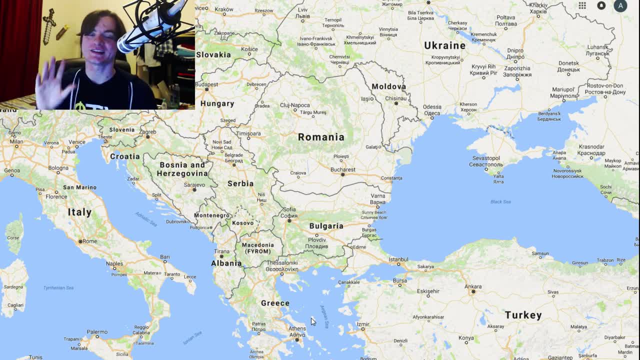 we've got that country right here. these six countries are like former Yugoslav countries. and then once you combine in uh, you know these countries right here, you get the Balkans. so there there's your Balkans, that's generally known as the uh. again, it seems rude to. 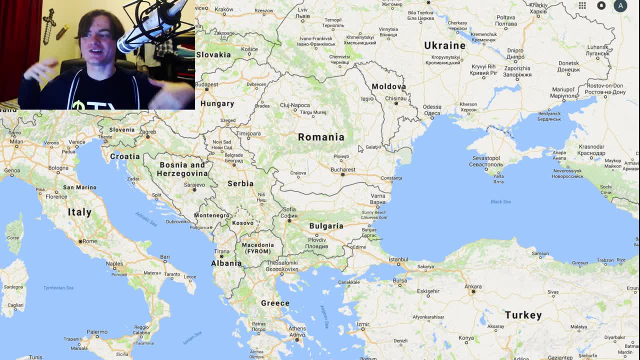 call something the less pleasant side of Europe, but that's where the, the war and the danger and the all this stuff was most recently. uh, one of the most recent wars in uh memory was the Kosovo War in like 14 years ago. 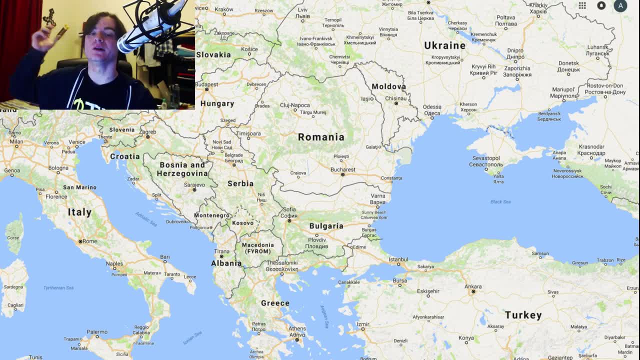 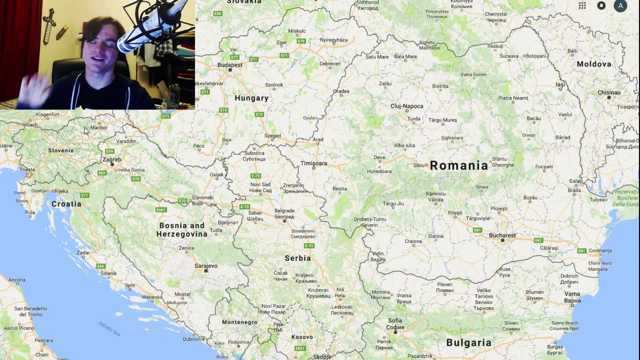 There's a lot of uh unpleasantness attached to this, but it is a very lovely place too. it's got most of the lovely sights. uh, you know, there's a beautiful lake in uh Slovenia- I forget what it's called- um beautiful lake in Slovenia somewhere. I uh Lake Bled, maybe. 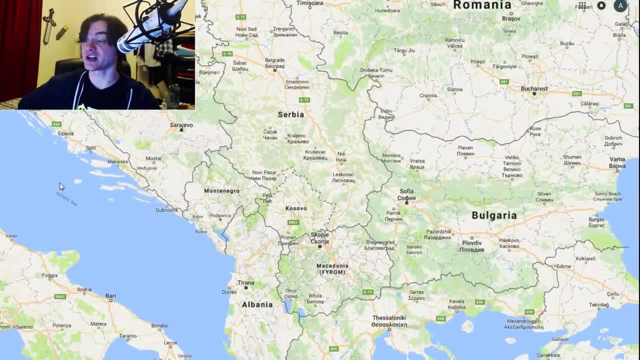 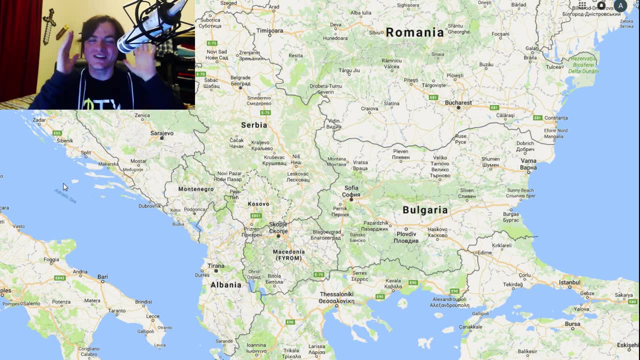 uh, there's a beautiful uh lot of geography and uh beaches in Croatia. it's very well known for that. there's a lot of beautiful stuff going on here as well as uh. by the way, my phone started ringing. I was like: uh stop, you know, trying to do geography. 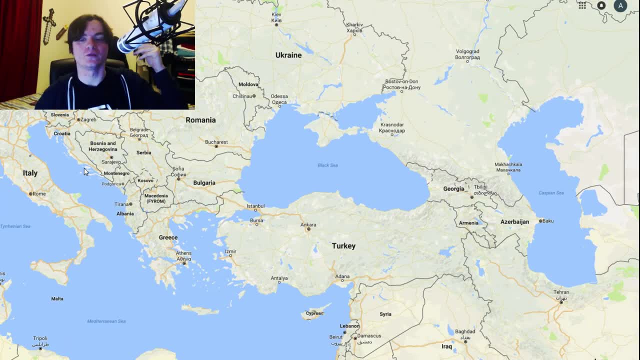 to the internet, um, but yeah, it's. it's got loads of beautiful stuff, it's got loads of beautiful culture, people et cetera, but it has that kind of bad reputation of like that's where bad stuff happened most recently. 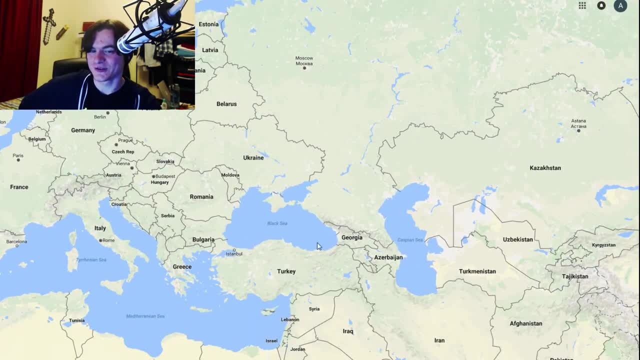 So yeah, once we've covered the Balkans, the Southeast Europe is like again, it also includes this stuff. uh, then we've got Far Eastern Europe, so like Eastern Europe is generally just saying anything, that was a former USSR state, so you've got your Ukraine. 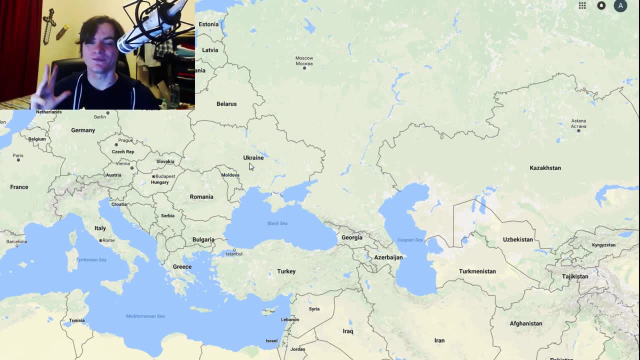 there you've got Moldova, which is the poorest country in Europe. Ukraine's actually the second poorest. um, again, you might, you might be like: why are you just calling out being poor? Well, it's this, it's the kind of you know. show you or explain to you the key difference. 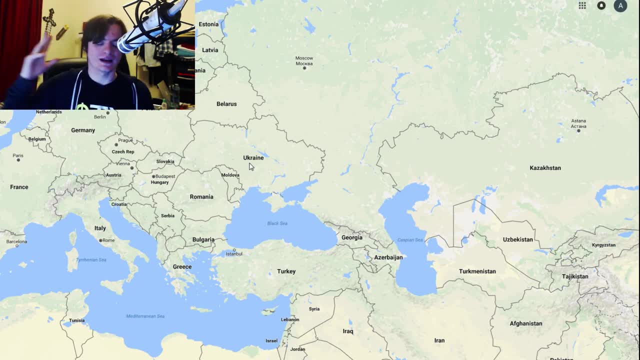 between like a Moldova and a UK is way more than the difference between like a Mississippi and a California. It is on a whole nother level. it's different between you know, like an African country and like you know Germany or something it's. it's that kind of level between Moldova. 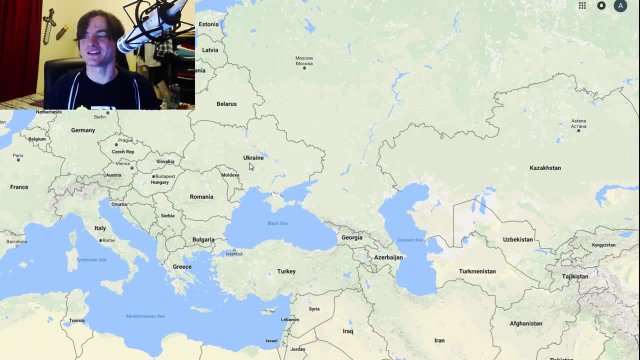 and the UK. so or, like you know, Moldova and Spain, let's say, because I'm from the UK, so I don't want to don't use that as an example. but yeah, uh, these, these, this. 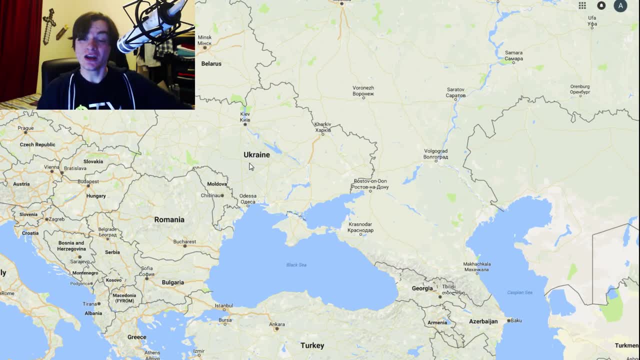 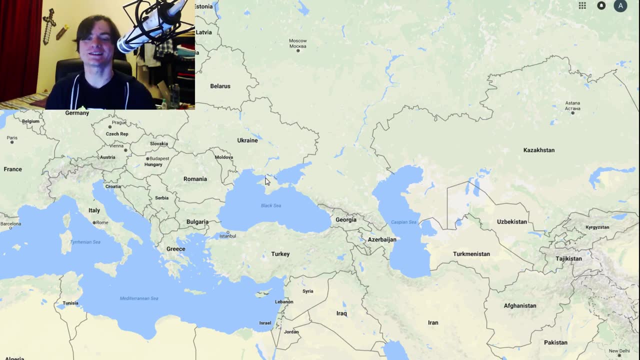 is kind of the the very destroyed part of, uh, you know, Europe by communism. communism did okay for certain countries, but it destroyed certain other ones and uh, yeah, there are some examples you can see in Eastern Europe here, as well as that, we've got Belarus. 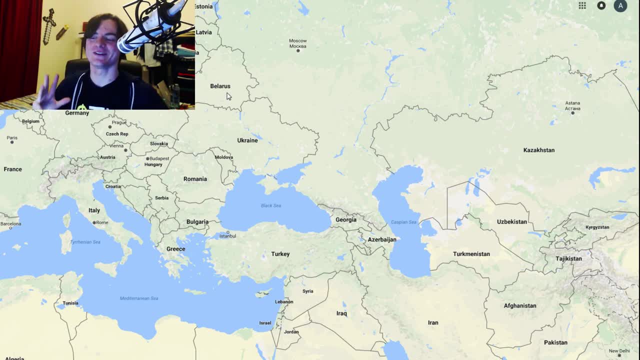 Belarus is kind of known as like the part of yeah. so again, Belarus is like one of those countries, Europe, that's very, very unwilling to integrate with the rest of the the West, uh, you know. 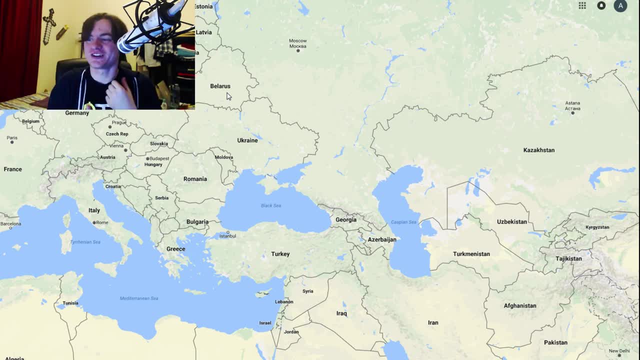 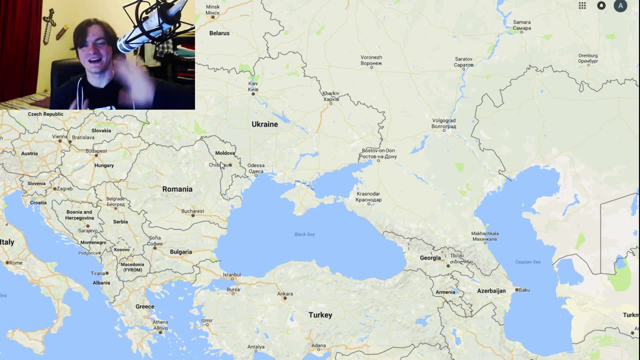 like Ukraine's kind of torn, but Belarus is firmly on the side of like Russia, Russia, Russia, Russia, Russia and uh, yeah, they're one of the only former USSR countries that are like that. We've got Moldova here, which is a split off of Romania. uh, lots of stuff to do with those. 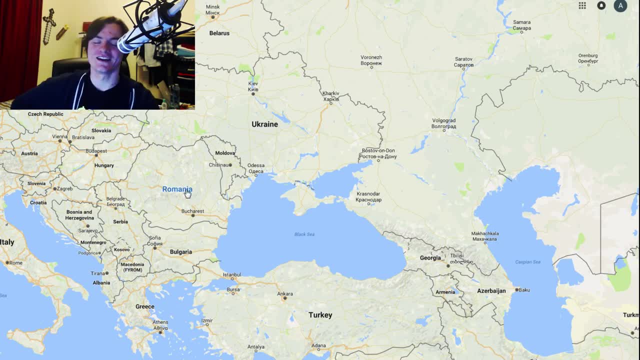 two countries and they're like: oh, come home Moldova. and they're like: no, uh, so yeah, that you got Romania Moldova. Moldova has its own split off region, I believe called Transnistria, which isn't officially. 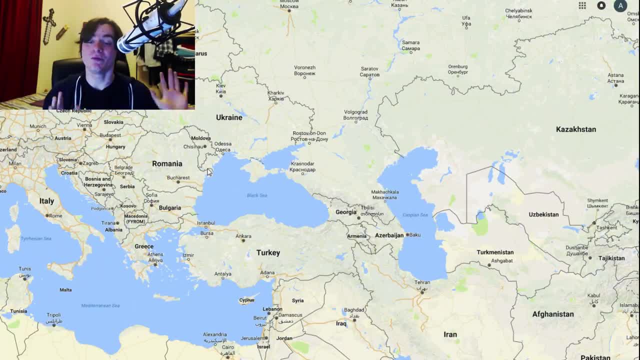 recognized, but it is its whole own country too. Again, there's lots of issues there, but once we've gone through that, we've got just one more region to cover. Which, oh, two more regions to cover? which is Central Europe? 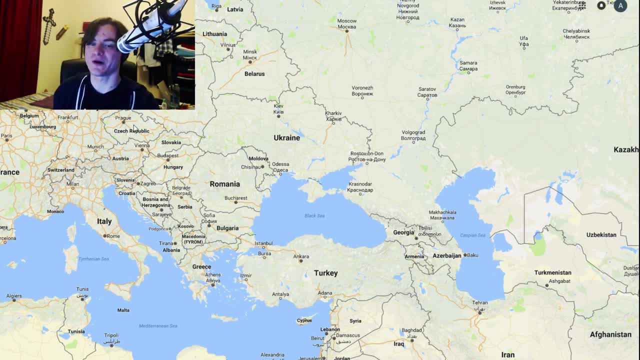 So Central Europe is again what they all like to call themselves. there We've got the Czech Republic, Slovakia, Hungary and Austria. Central Europe is kind of like not really east enough to be called East Europe- even though they were former USSR countries in some cases- but not really west enough to. 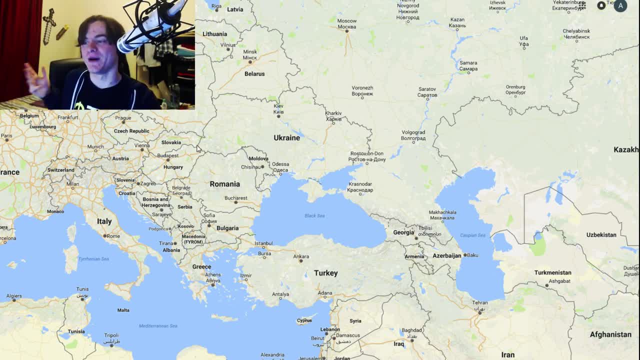 be called um Western Europe. you know you wouldn't call Slovakia Western Europe. So, uh, yeah, Central Europe is what they generally call themselves, sometimes along with Slovenia, and uh yeah, these are the countries right here. 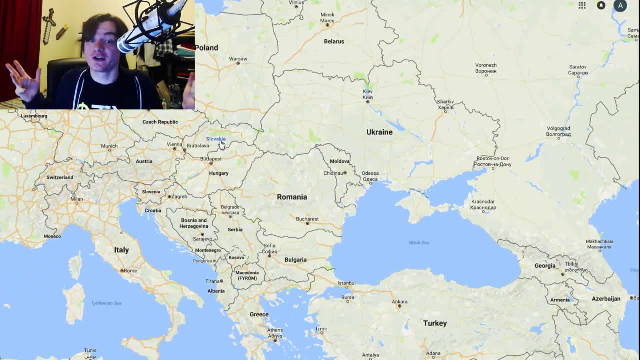 Uh, in particular, Czech, uh, Czech Republic and Slovakia, and you probably don't know them by those names. You probably know them as Czechoslovakia because they used to be. they used to be best friends. They had one of the nicest divorces between two countries, but that is Czech, uh, Czech. 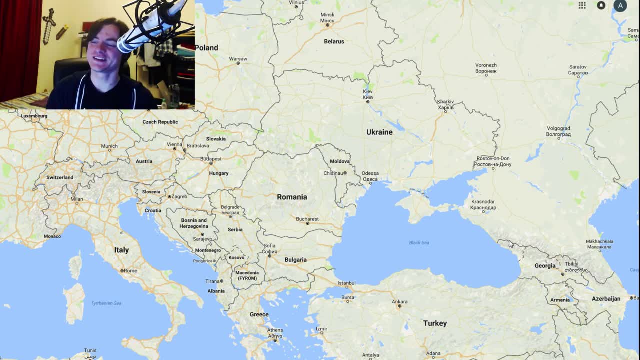 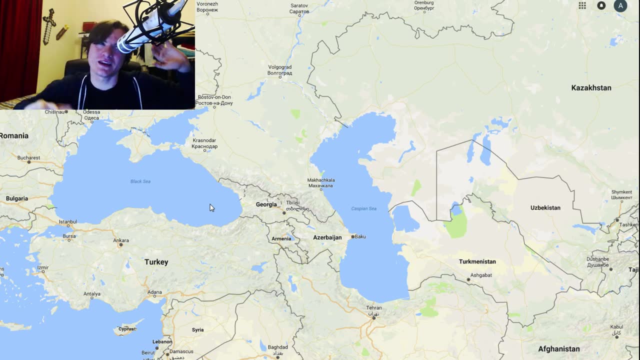 Republic and Slovakia, And then finally, I'm going through every European country today, but we're gonna do this Um. then finally, we've got the- uh, the countries over here, which is the Caucasus region. So this is um, again it's uh, it used to be USSR, so again all those connotations. 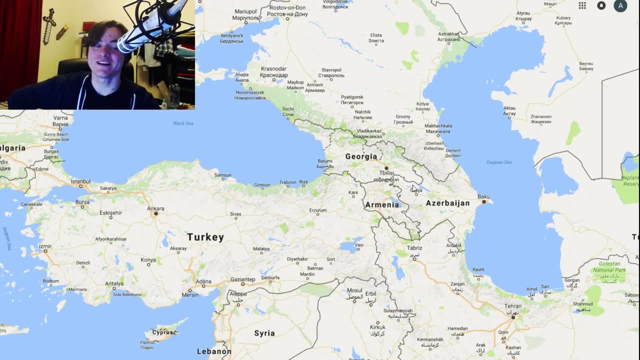 Uh, and also they've got loads of breakaway regions. There's lots of stuff going on here, but there's three countries. You've got Georgia, you've got Armenia, you've got Azerbaijan. So Azerbaijan- um, if you have played your video games, 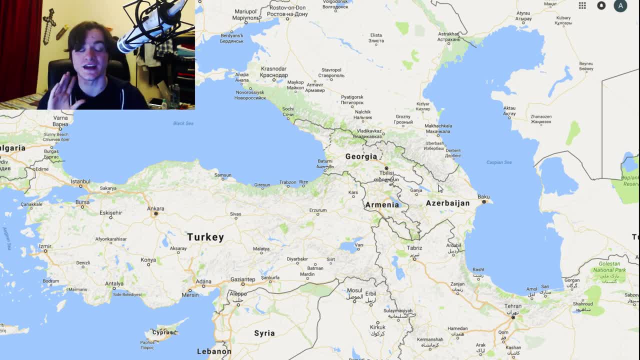 is where I I think it's one of the more famous segments in uh Call of Duty 4.. Uh, Georgia, I know, is uh very, very it's. it's probably the most visited out of all. 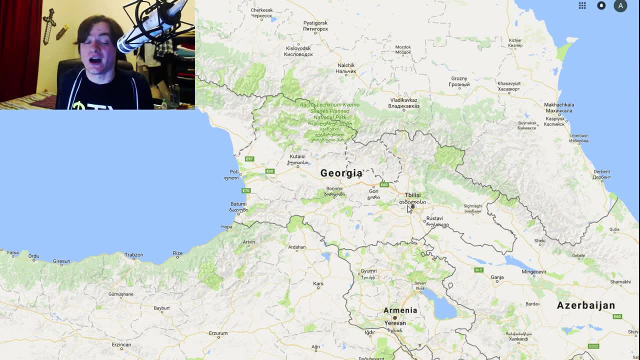 of these and I know it's, I can't even pronounce their capital. I'm sorry, Um, but I I know that's, uh, again, an incredibly lovely place that lots of people recommend and stuff. Uh, if you want to go to somewhere, that's kind of out there but not all the way out. 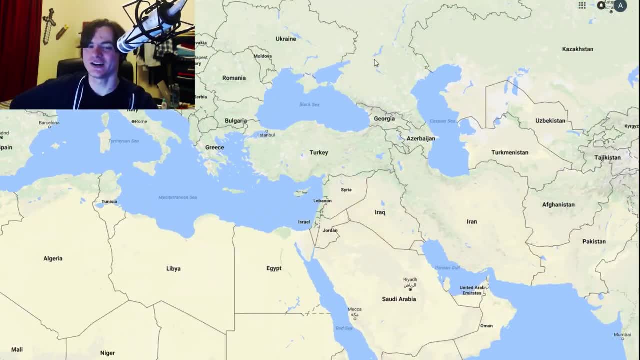 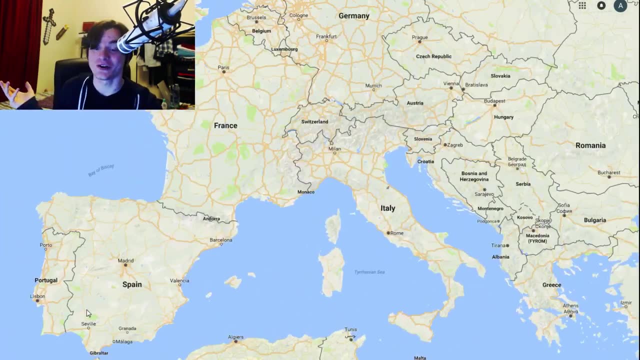 there, uh, Georgia is one of the places that's known for that. And yeah, long story short, Europe big place, Lots of stuff going on. You can't really call Georgia and Azerbaijan, uh, the same places as you can call Portugal. 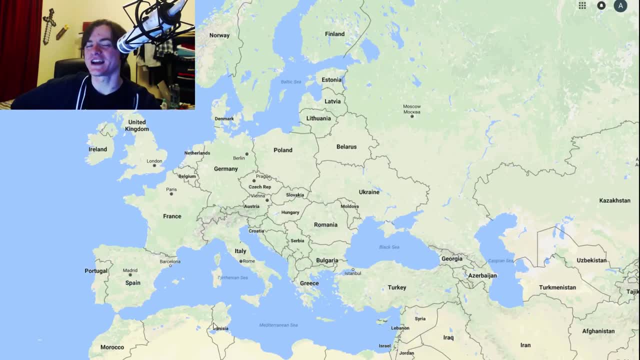 As it just so turns out. And um, also, by the way, one more thing. I guess you can kind of count islands. Uh, there's really only like the UK and like you got Malta down there and you got. 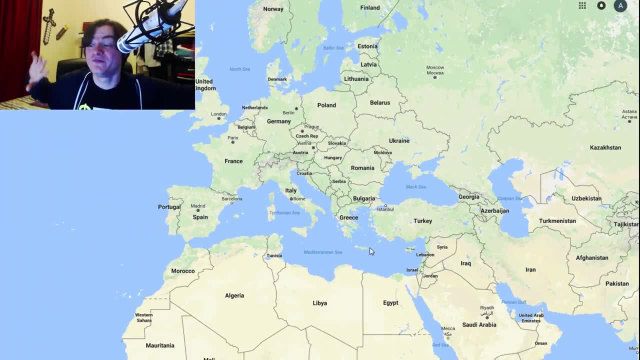 Cyprus and you got those countries like that. But uh, yeah, there's your vague regions of Europe. Now you know, You got your to go very, very briefly through them again. so you're like: okay, this, this. 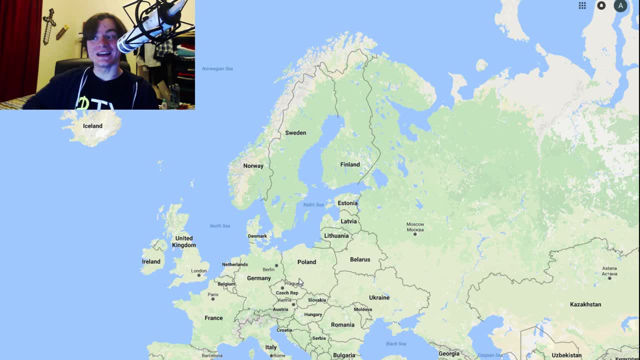 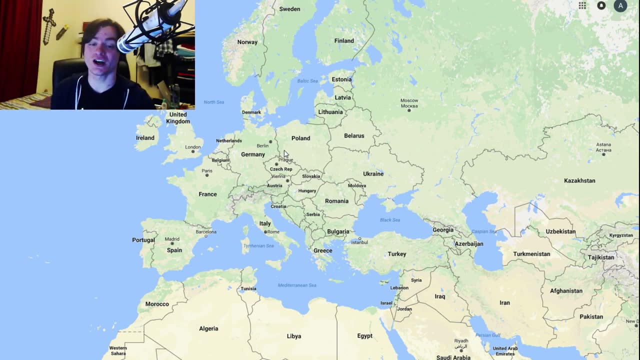 that. Uh, you got your Scandinavia, which is like your. hey, I am from Scandinavia and I am very friendly. You got- okay, we're doing horrendous accents to go with this- You got Western Europe, which is the Europe you probably picture with your Amsterdam. 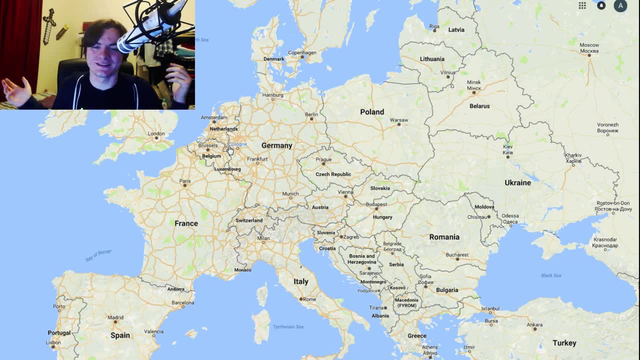 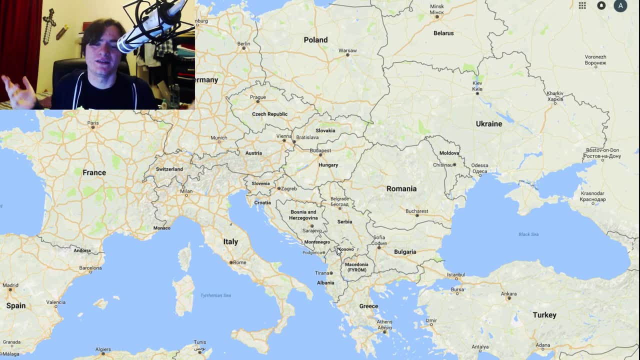 with your Paris, with your your Frankfurt and your Brussels and your London. Uh, you got that in Western Europe. Then if you go to Southwest Europe, you get the the kind of more conflict ridden, but now again it's a lot better than it was at some point. 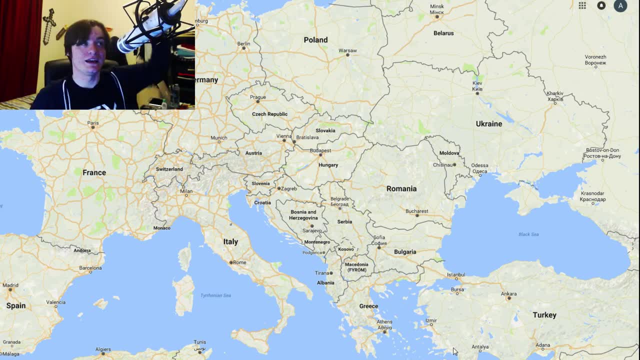 Uh, you got this kind of side right here. You've got Eastern Europe, which is generally known as being poor. Again, I don't, I don't have like the correct term for like a country with less collective. 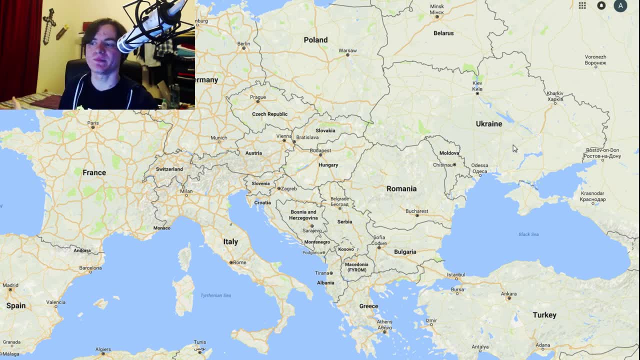 wealth is, but the generally poorer side of Europe, which is over here, where things are a lot cheaper, uh, but the country is doing slightly less well off, Uh. then, finally, we got the Caucasus, which is only part of Europe. 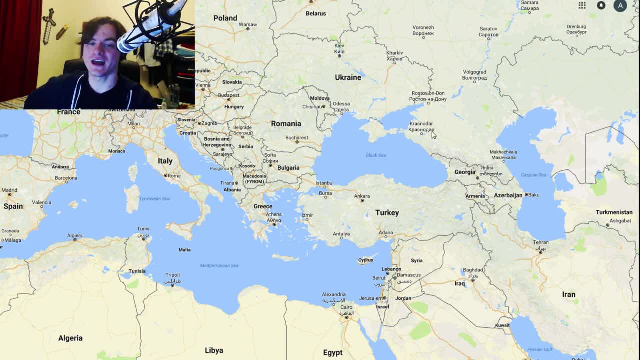 By technicality, because it's like all the way out there, but again separate thing over there. Uh, ex-USSR countries. And then finally you got the Baltics, who are just like, yeah, we love you Europe. 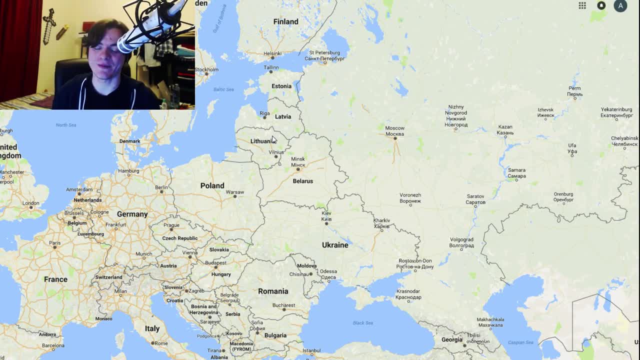 Thank you for saving us. Please don't hurt us. Russia, And uh, maybe, maybe that's too much. uh words from one video. Maybe you didn't understand any of that, And if that is the case, then I'll let you know that I got a new water bottle. 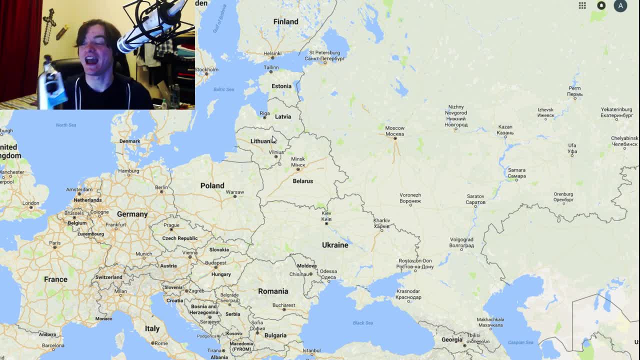 So it's uh, stainless steel, uh something, something, something, And uh, I, I, I like it a lot better than the old one, because my old one would leak And uh can totally recommend if you need to drink a lot of water like I do, because 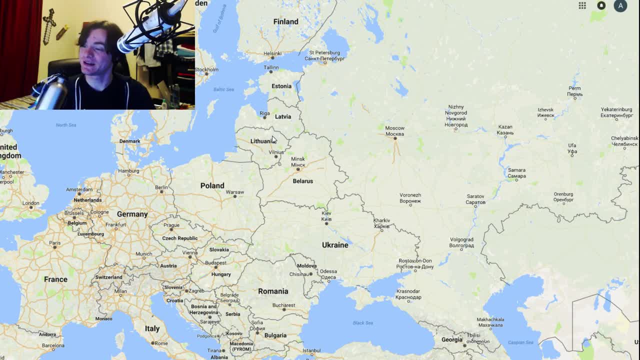 I talk so much Do the things with water that you should buy one of these because, or just a water bottle in general, Because one I, I mean, I, I it kind of looks cool but also like it retains the. 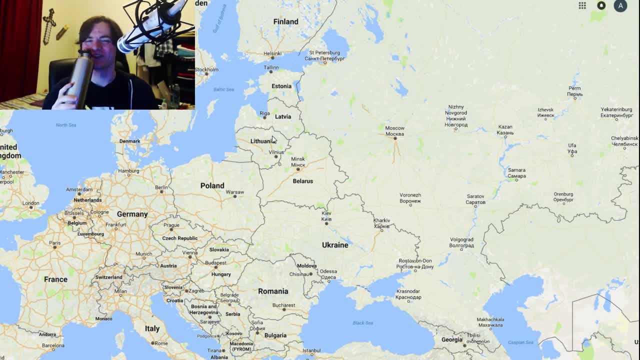 heat so well Like this is still cold, even though I'm like sweating right now, So useful. I hope you enjoyed the video. Uh, make sure you check out the rest of the Geography with Toy Cat playlist If you want to see videos that are much less short. 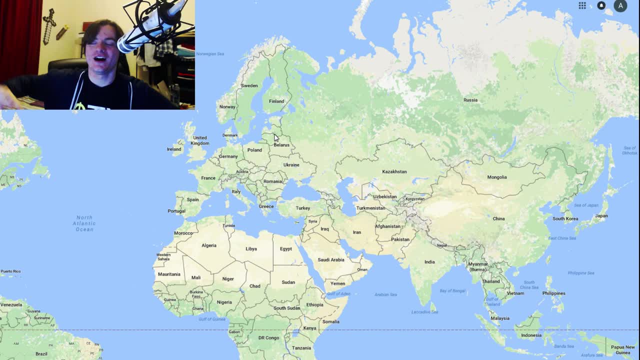 Um, do you want to see more uh videos like this about other parts of the world? Let me know. Uh, I don't know. Uh, thank you very, very much for watching, though, And I'll see you all next time. 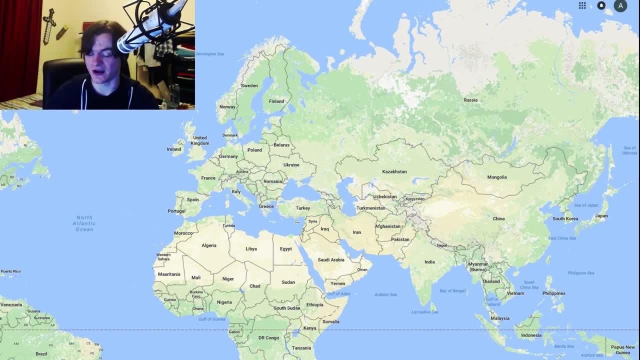 Goodbye. I don't know whether this I need to. I need, I need to set up a, a, a like a hotkey for stop recording, Because I know there is one, but I don't know what it is. 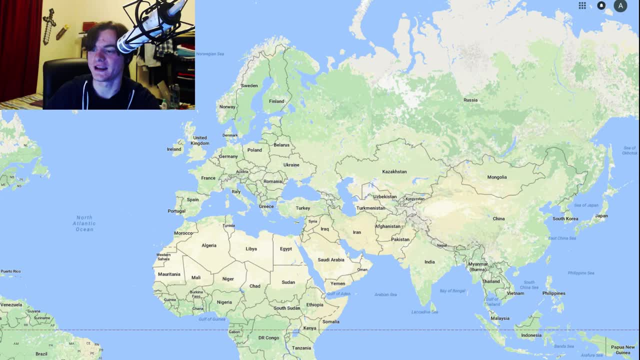 So I'm going to try pressing F8 right now. That was not the hotkey. Okay, stop recording. 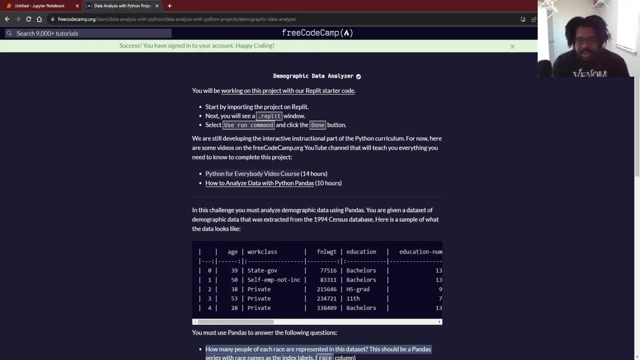 all right, boom. so welcome back to another video, guys. today what we're gonna do is we're doing the demographic data analyzer for free codecams: data analysis with python. so in this challenge, what we must do is analyze our demographic data. using pandas, we're given a data set of demographic data.